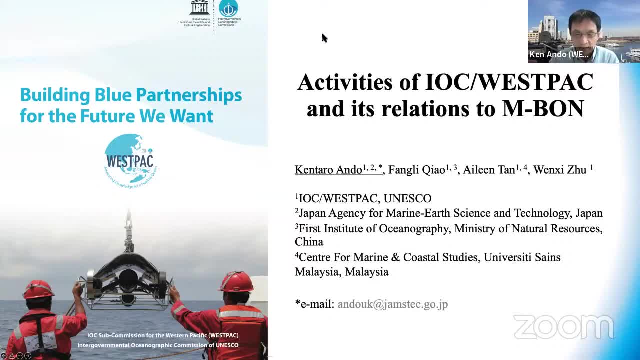 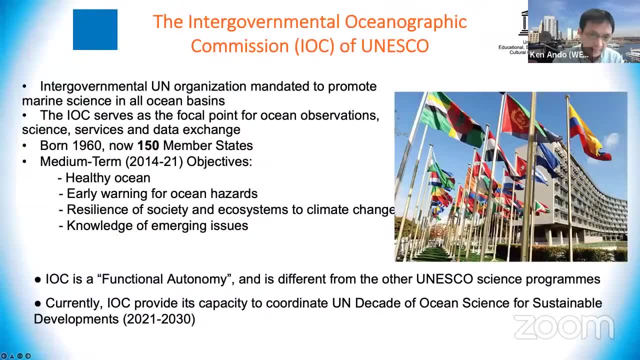 Char and Eileen Tan and went ZZU. Uh, I'm not sure they are here, but uh, Dr, they are the officers and secretariat of IOC Westpac Dr. So let me first introduce about the IOC Dr. Uh, IOC is the intergovernmental. 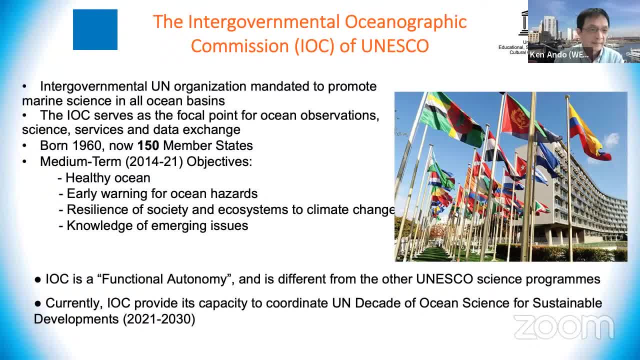 an organization mandated to promote marine science in all ocean bases. IOC serves as a local focal point for ocean observation science services and data exchange, And IOC was born in 1960s. Now we have 150 member states, And now so it is already over. but 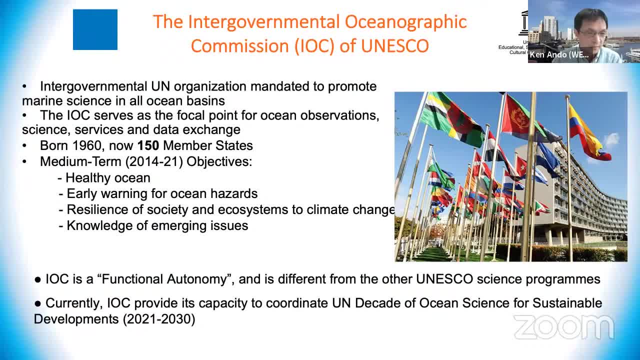 we had four objectives: healthy ocean, early warning for ocean hazard, resilience of society and ecosystem to climate change and knowledge of emergency issues. And IOC is functional, autonomy and different from the other UNESCO science program. Currently, the IOC provides its capacity to coordinate UN Decade of Ocean Science for sustainable development. And IOC 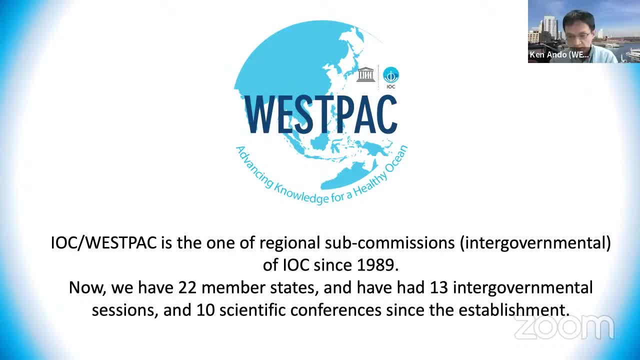 provides its capacity to coordinate UN Decade of Ocean Science for sustainable development, And Westpac is one of the regional subcommissions of IOC since 1989.. Now we have 22 member states and have had 13 intergovernmental sessions and 10 scientific conferences since its establishment. 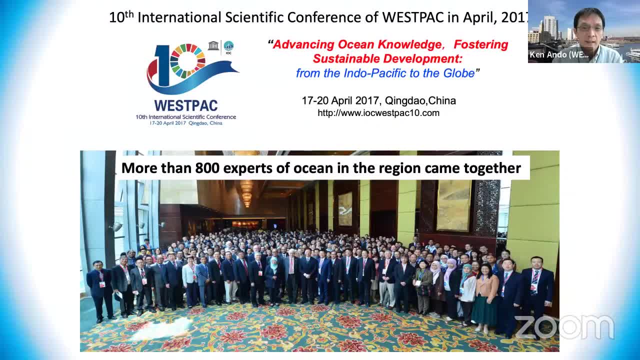 And this is one example of our activities- We conducted a 10th international scientific conference in April 2017.. That was taking place in China, Qingdao, in 2017.. And we planned to have this kind of activity in 2020, but due to the COVID, we have to postpone these activities And 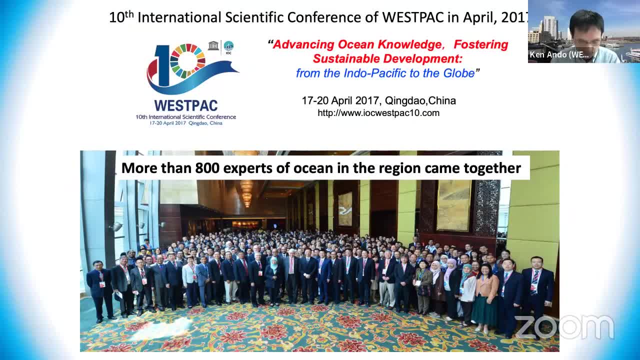 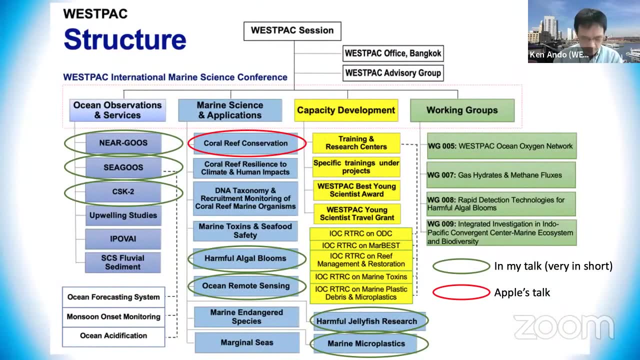 we are planning to conduct this conference this year or next year. For this conference in 2017, more than 800 experts were gathered. So these are the structures of Westpac, And at the top we have the Westpac session And we have an office in Bangkok And under these, 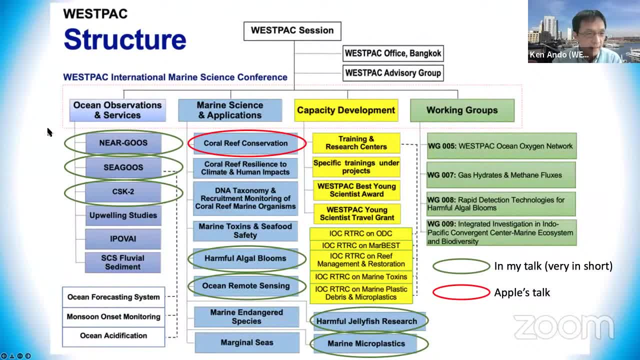 activities. we have 16 activities grouped in a group, So we have a lot of activities And at the top we have the Westpac session And we have an office in Bangkok And under this school of operation, which started in 2005,, is our account administrator. So we 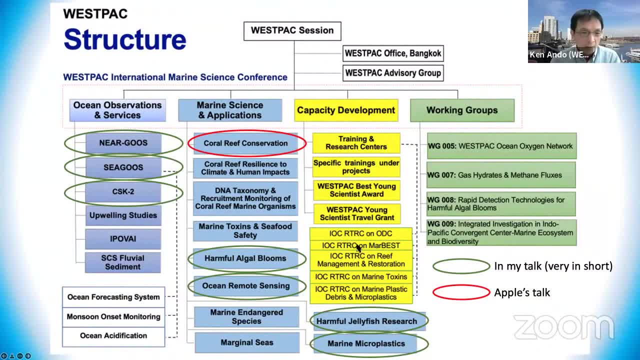 are going to do a virtual workshop in Kent, so we have that virtual workshop on YouTube or Facebook, But may be some of you have already assembling a unit to work with this institute, But I don't know what's the best time to be giving themselves an audience's. 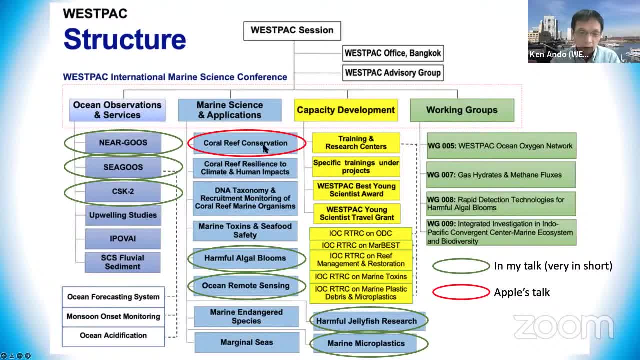 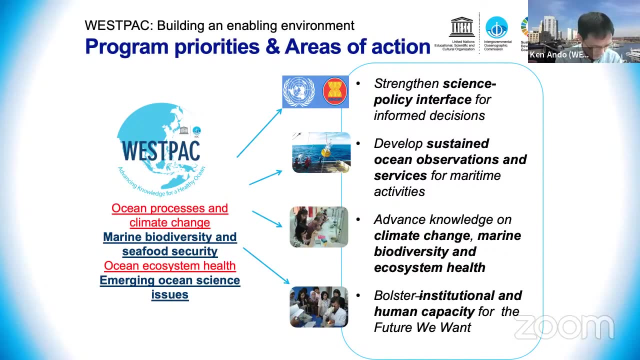 speaking around. our contribution to the research Goal 6,, for example in the World devotions webinar, Were horizontal park surveys at bm-stateorg Sh? vê. xì, xè, xè, xè. respect priorities and areas of actions. We have trying to conduct the researches. 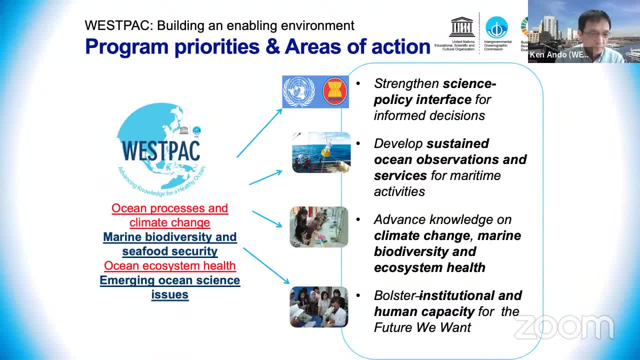 focusing on ocean processes and climate change, marine bio-diversities and seafood securities, and ocean ecosystem health and emerging ocean science issues. To do so, we try to strengthen science policy interfaces and also develop sustained ocean observations and services and also advance knowledge on climate change. 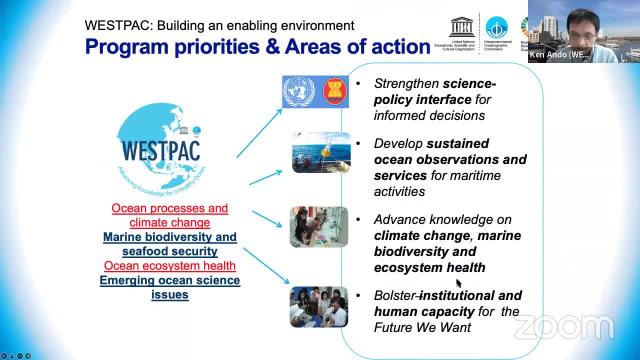 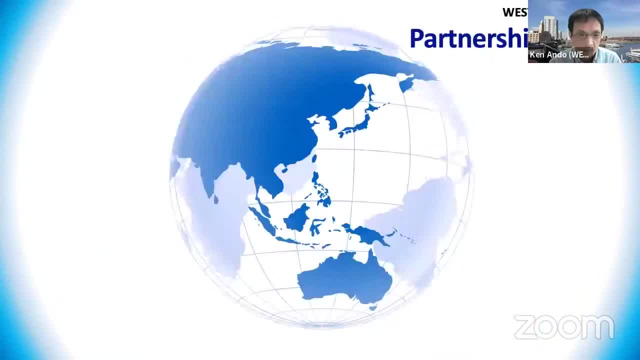 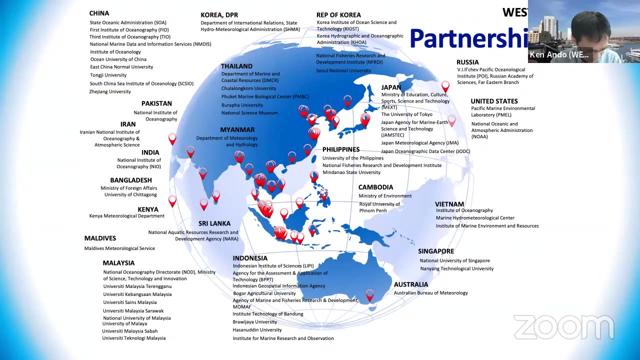 marine bio-diversities and ecosystem health And finally, bolster institutional and human capacity for future we want. Currently we have many partnerships in this, mainly focusing on in these regions. So you see, we have a lot of partnerships in mainly focusing in these regions. 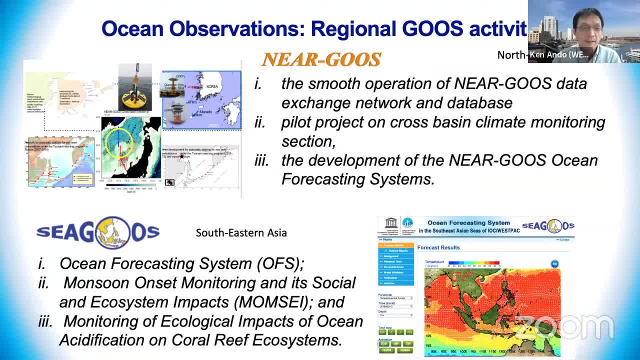 So let me introduce one by one about our activities which I think related to the biodiversity observing networks. One is about ocean observations in these regions. Now we have two regional GUCCIs under Westpac activities. One is near GUCCI, focusing on the northeastern. 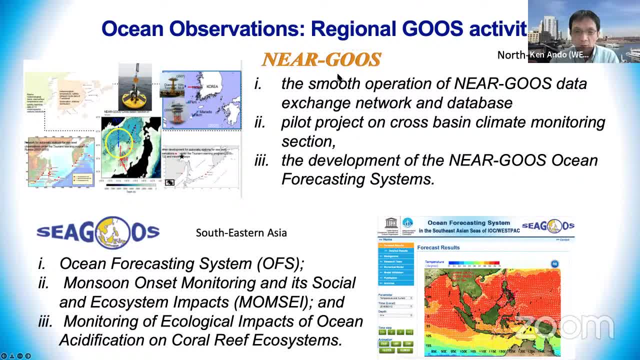 and the west of Asia And they are going to conduct a smooth operation of near-GUCCI data centers And also conducting the pilot project on close-basin climate monitoring section in the Sea of Japan And also develop the forecasting system- ocean forecasting system. 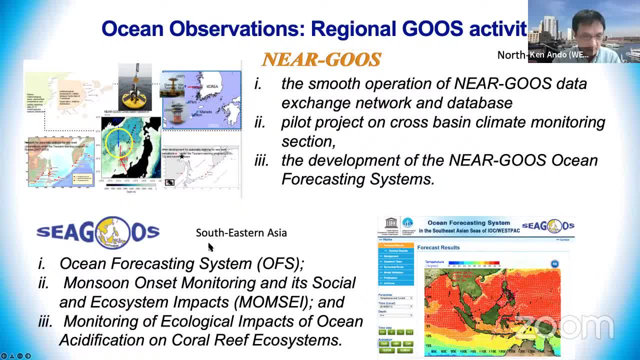 We have another regional GUCCI, named Sea GUCCI, focusing on the south coast of Japan and the east coast of Japan- Southeast Asia. In this regional booth they are also conducting ocean focusing system and other observational activities on sea and also the monitoring of ecological impact of. 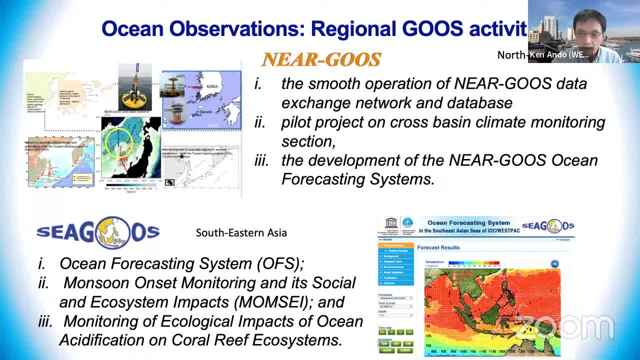 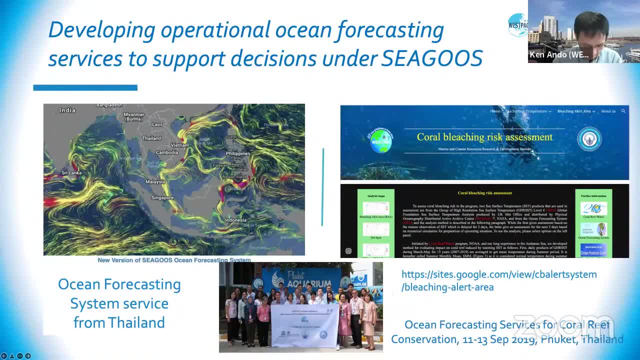 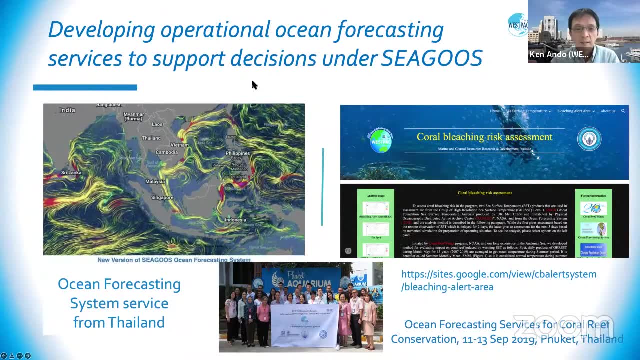 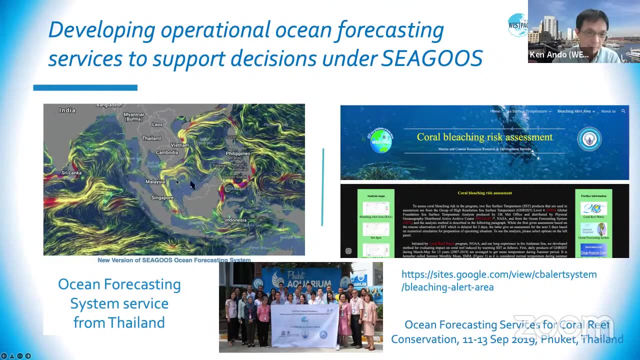 ocean acidification. This is one example under the sea booth. So the ocean forecasting system team is developing the operational ocean forecasting services to support the decisions under the sea booth. This is the animation developed under the sea booth And also they are conducting the 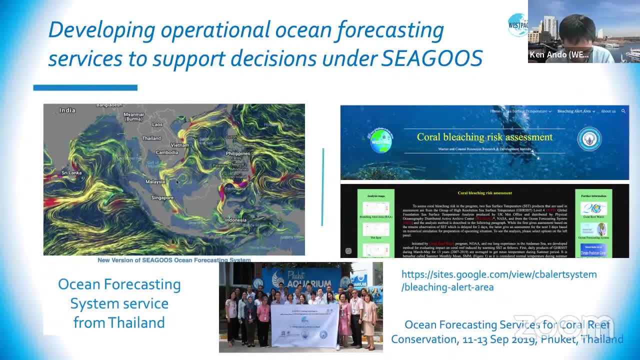 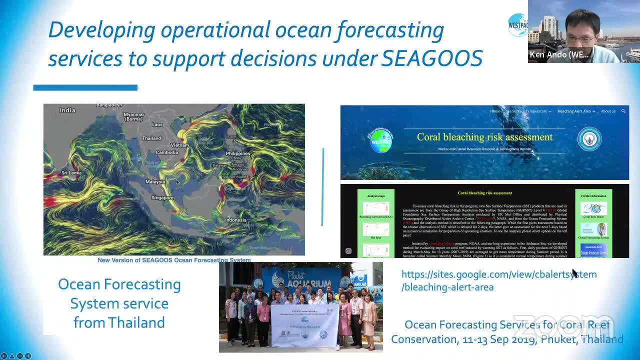 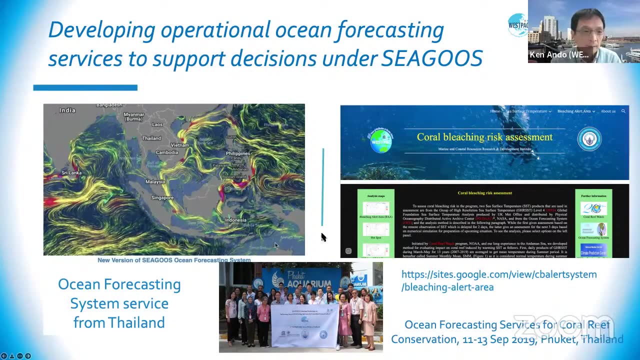 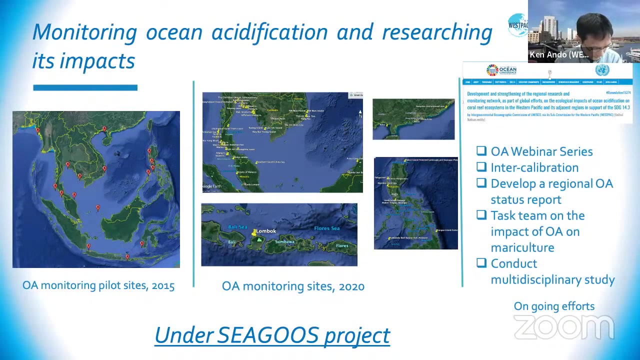 by using the model output, they are conducting the coralline reaching risk assessment And also they are conducting some workshops focusing on their ocean forecasting services. Next one: Okay, So this is also another example by the leadership of experts in Thailand. 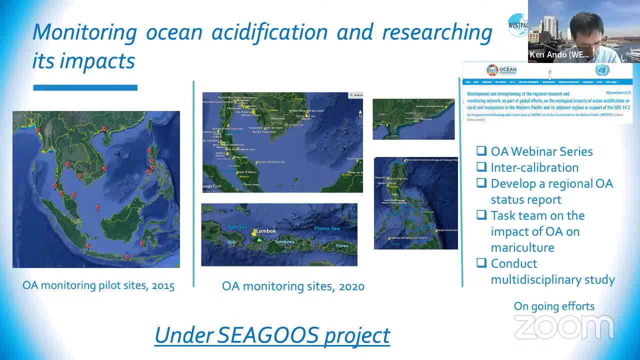 Westpac Sea Goods has developed the observational network for coastal ocean acidification. In 2015, here we did not have so many coastal stations for ocean acidification, But now, in 2020, we could have more stations in coastal of our regions During the periods. 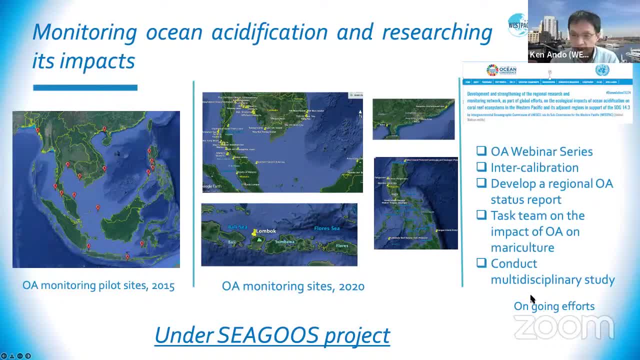 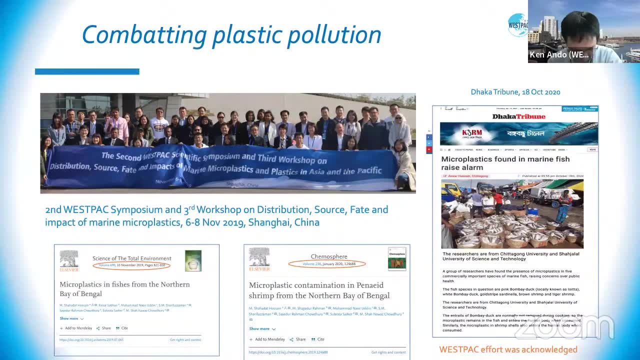 we had webinars, intercalation exercise, regional, you know report, something like that. Yeah, And another project under the Westpac: marine plastic pollution has now become big issues for marine environment. Westpac established the marine plastic pollution project in 2017.. We conducted several workshops to share. 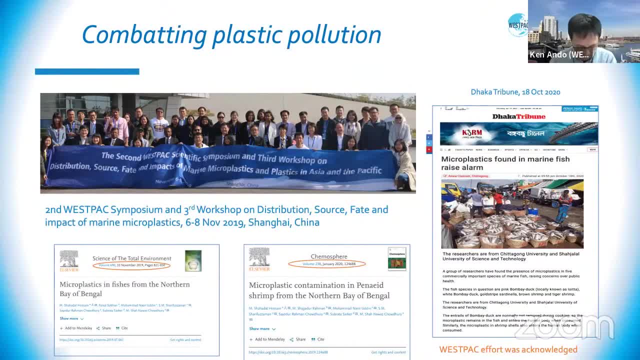 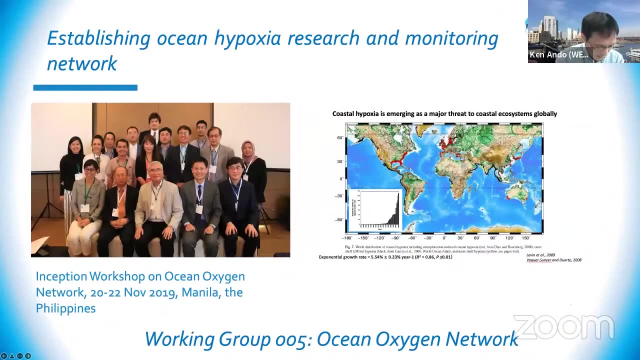 information knowledge and to have better plastic science for solutions to society. An expert in this project published papers in which Westpac was analyzed, And it was also the project that led to the implementation of the Ocean Hypoxia Project. The project was developed by the затем Austin Research Program in May. 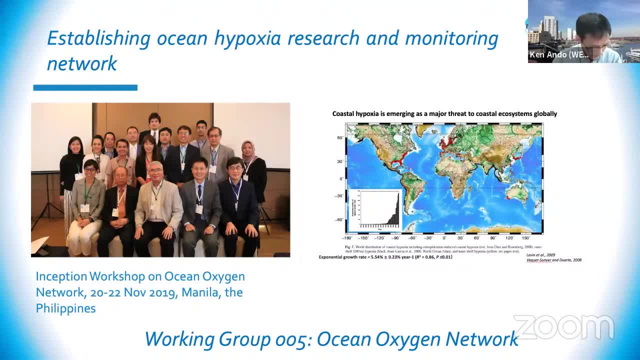 as an end-to-end discussion about the impact of the ocean. Ocean Hypoxia causes a variety of impacts on ocean ecosystem, which requires oxygen for productivity and provides services that sustain people's livelihood. aspects of deoxygenization and help inform policymakers on the issues for decision declining. 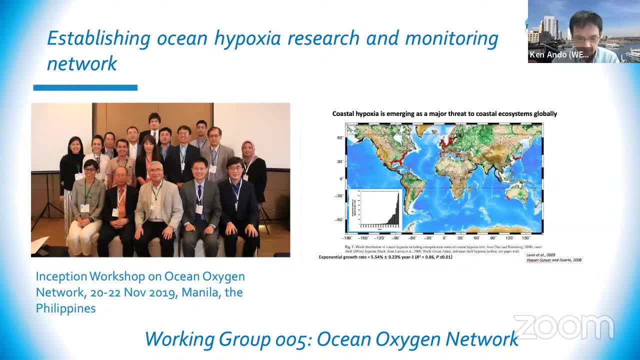 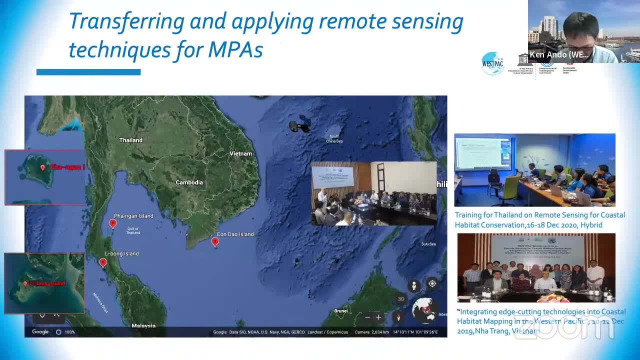 oxygen in clear coastal and open waters. Remote sensing has become an important tool for the managing of marine environment and for mapping marine habitats. To promote its development and application in this region, Westpac took demand-driven and solution-oriented approach to the development of application of remote sensing techniques. 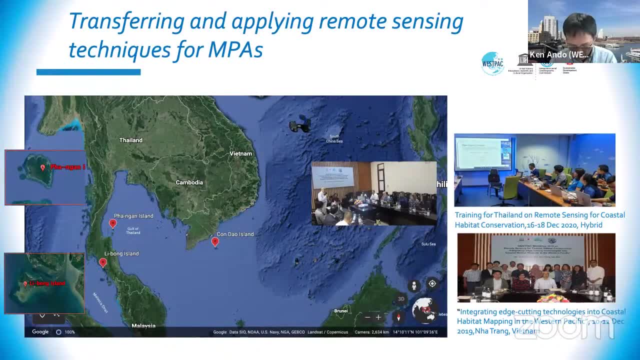 In close communication with national or local authorities, Westpac selected three MPAs- Ribbon Island, Pha Ngan Island in Thailand and also Khon Dao site in Vietnam- as a pilot site. These MPAs were developed based on their needs and started to transfer relevant technologies. 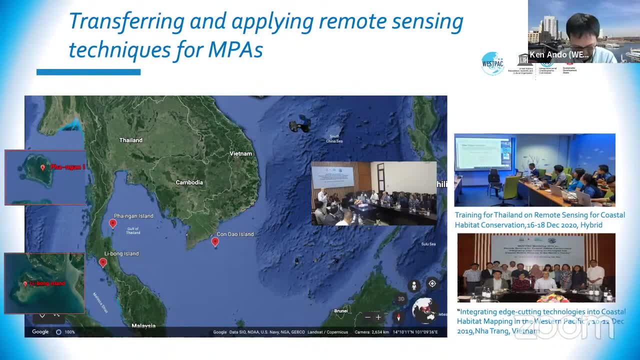 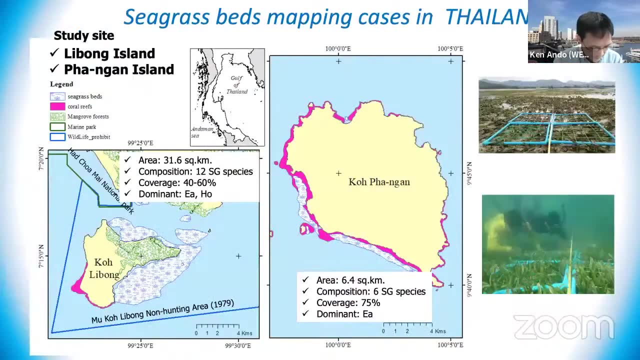 of remote sensing and assisted in producing sea-glass mapping for marine protected areas management. This is the enlarged plot of mapping site in Thailand by Westpac Ocean Remote Sensing Project. I'm not an expert so I cannot go into detail, Sorry. 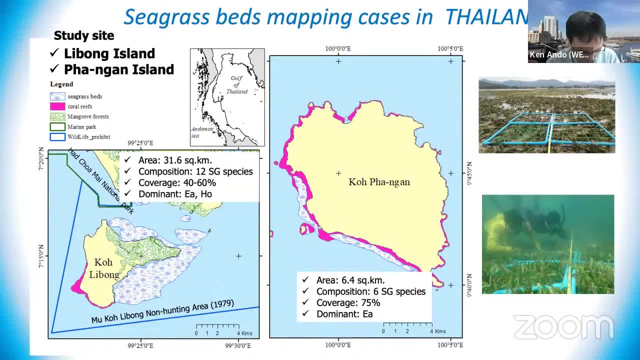 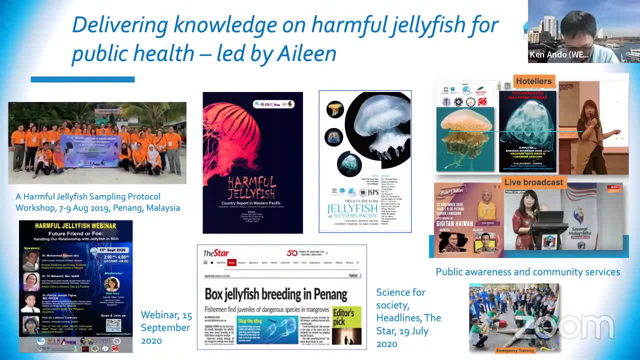 But it's a great project, Thank you. Thank you. Thank you for the introduction and I'm sure you will continue to be interested in and try to conduct in situ observations. Jellyfish invasion in Westpac country is becoming an emerging treat to humans as more and more. 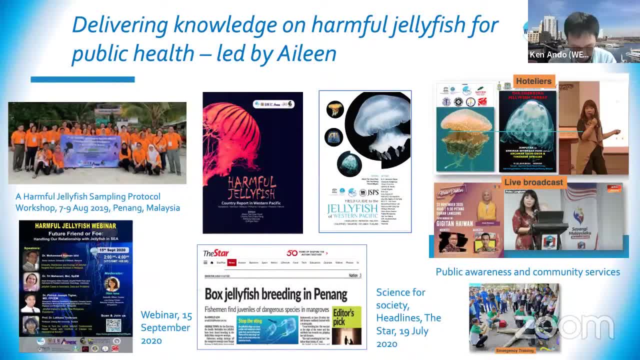 cases of jellyfish stung have been reported. Jellyfish have brought havoc on turkeys industry in coastal areas. Since the establishment of regional harmful jellyfish network, laboratory development has been increasing And this has also contributed to the colonization of seawater. 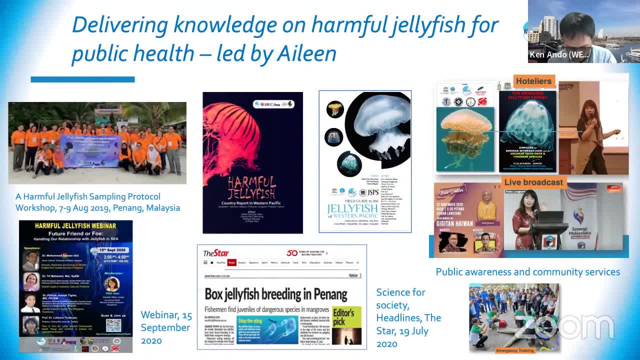 Network. in 2017, sub-commission has been coordinating the joint research on harmful jellyfish with field guide to jellyfish of Western Pacific published in early March 2021.. To raise public awareness, outreach and awareness activities on jellyfish bloom and emergency response. 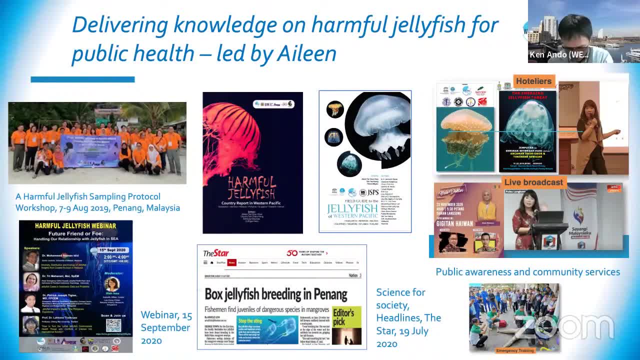 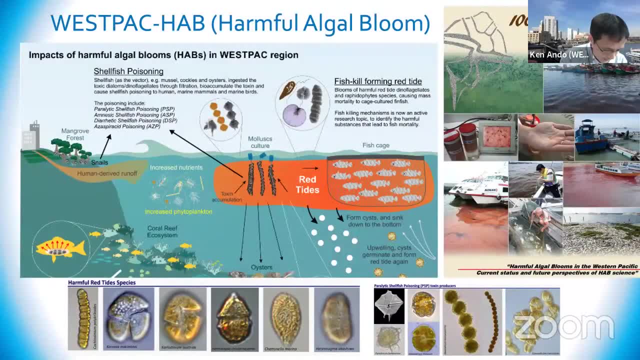 has been conducted for hoteliers, coastal government authorities and school students. The Westpac HAB Harmful Algal Bloom Project would be the most long-term project in Westpac and I think it started early 1990.. HAB causes shellfish poisoning and fish kill when it happens. 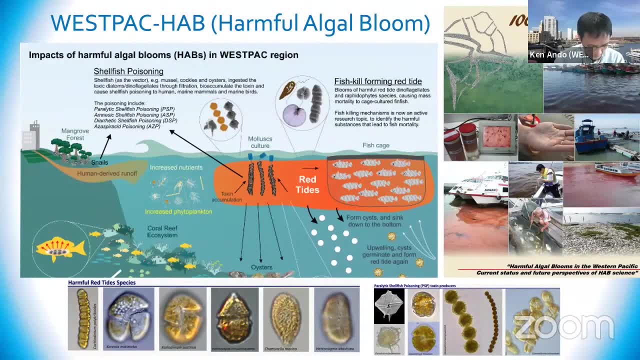 There are many species to cause HAB, so in-situ sampling is always important to identify its species. Westpac HAB project has published several books on the current status of HAB in the region, in the Asian regions, and has been contributed. 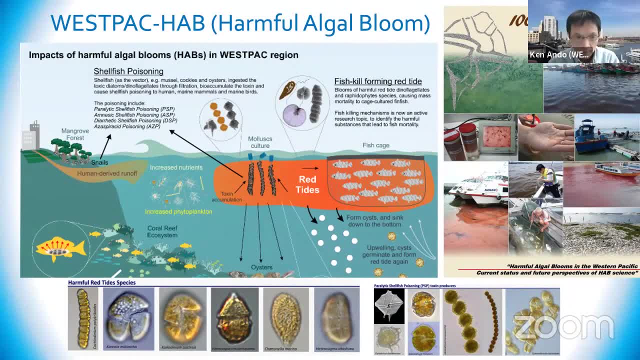 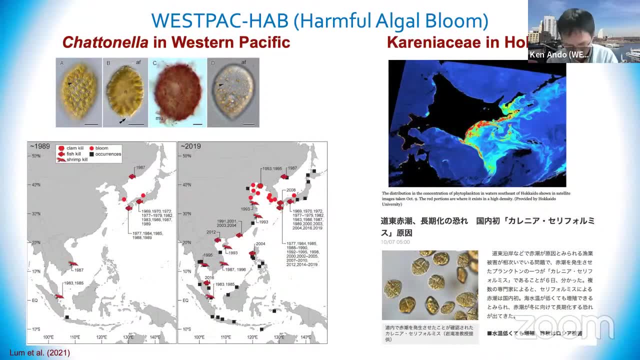 to the global HAB network. Recently, due to the emergency of ocean pollutions and eutrophic conditions in the coastal areas in Asia, HAB has now been highlighted to be occurred more frequently. The left map of HAB occurrence. this left map is the map of HAB occurrence until 1989,. 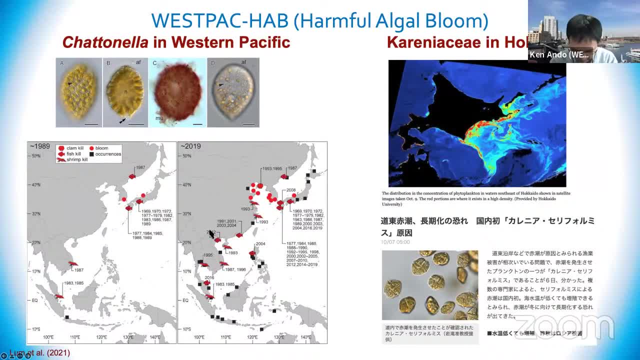 and this is until 1990.. It is clear that the frequency of occurrence of HAB is very low. It is clear that the frequency of occurrence of HAB is very low. It is clear that the frequency of occurrence of HAB is very low. 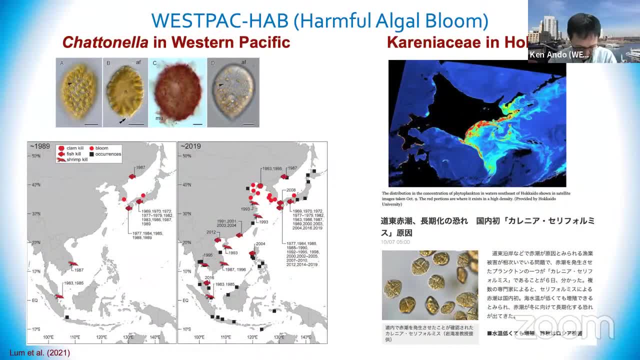 Recently, Japan experienced the occurrence of. recently, Japan experienced the occurrence of arugula blooms east of Hokkaido. in the last year, arugula blooms east of Hokkaido in the last year. In this case, satellite data could detect the concentration of 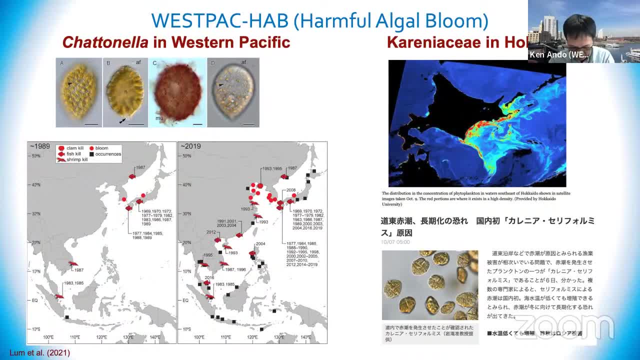 white plankton and by sampling seawater. species causing this bloom was identified: carinia. This bloom caused big economic damages, particularly in the Hokkaido Islands. Based on this situation, HAB project identified five directions of research. One is about the needs to identify co-saved species. second is the use of technical advancement. 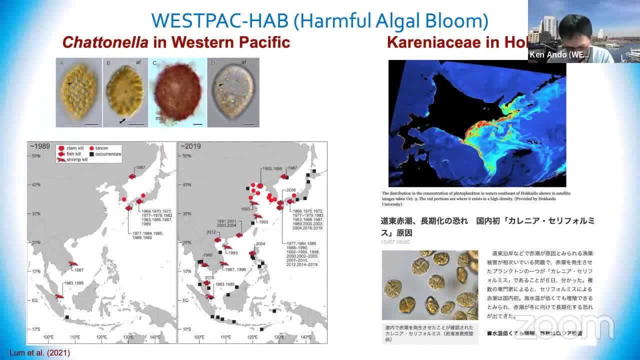 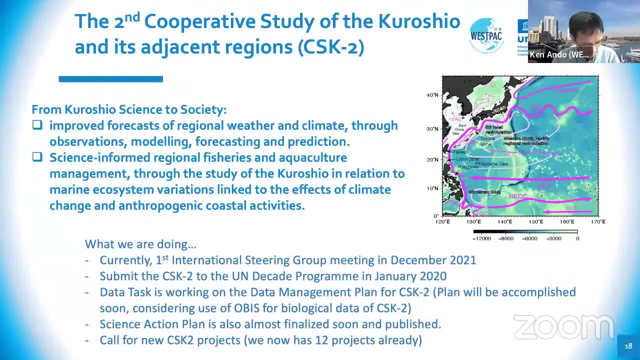 third is sharing good practice of monitoring. and fourth is advance of mitigation measures. And the final one is need to coordinate with other programs. In the last intergovernmental session, a new program was established, named CSK2.. This one, I myself am taking lead, focusing on the Kuro-shio science and also the society. 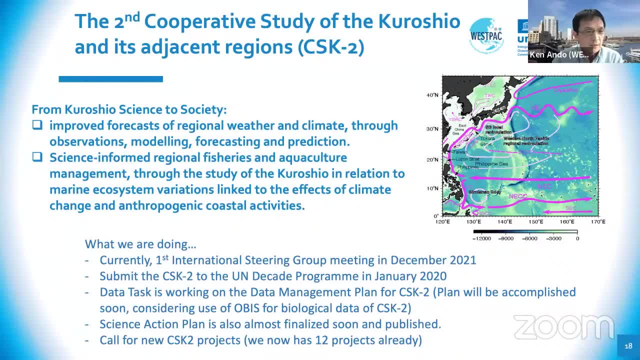 We have two objectives: one is to improve forecast of regional weather and climate through the observation, modeling, forecasting and prediction, And second one is the science-informed regional fisheries and aquaculture management through the study of Kuro-shio in relation to marine ecosystem variations linked to the effects. 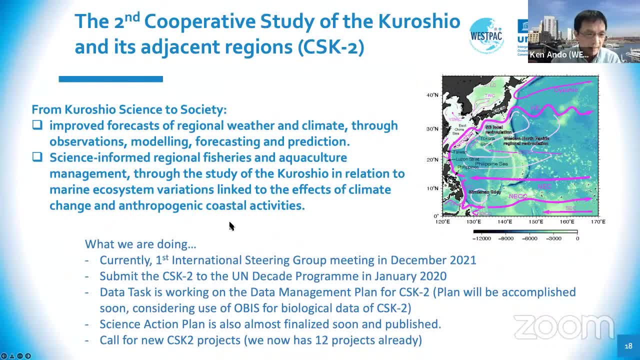 of climate change and anthropogenic coastal activities. Now we are doing currently: we conducted the first international study group and then we submitted this CSK2 plan to the UN. Thank you, Thank you. So in the next slide you can see how we designed the CSK2 project. In this slide. I usually explain it in Coveron's mobile, which was first easy, but finally I may Junglai and also ABA, please share with us later, while closely following the global emergency issues and also we try to conduct training. through research and also try to co-design and co-develop with member states of westpac and try to promote south and south and north to south cooperation. so this is the kind of the strategy of capacity development and let me show some examples. uh, this is one of activities of westpac. 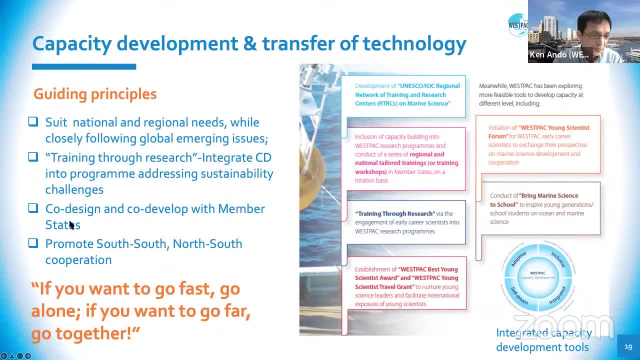 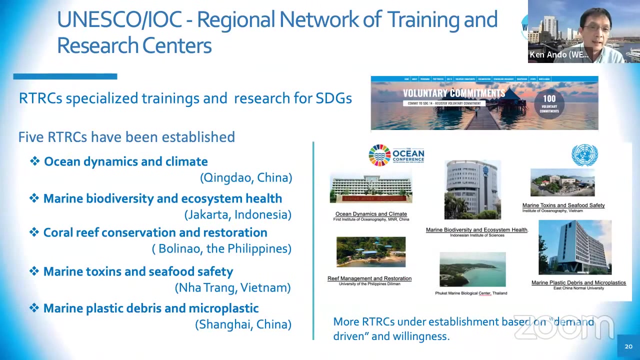 named regional network of training and research centers, so we try to establish the rtlc- regional training and research centers- in these regions. currently we could establish five rtlc's among five alternatives. first two, you know, the ocean dynamics and climate and marine biodiversity and ecosystem health has been, uh, you know, conducted in china and also in indonesia. and other threes: 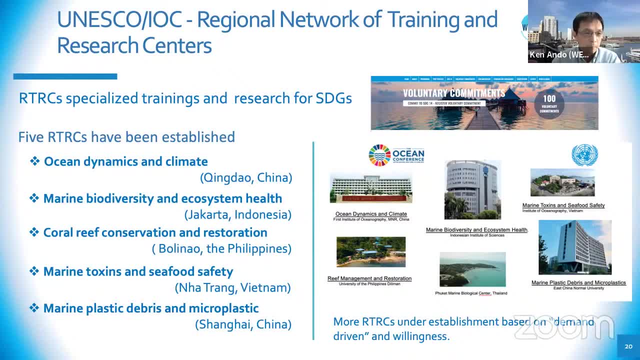 have just finished its feasibilities and waiting for the- you know green sign from the ioc palace. and also we recommended it to all westpac programs to conduct training workshop in their capacity and also encouraged to our member states to support to conduct training sessions, for example, in 90 2019, harmful rice based marbles. 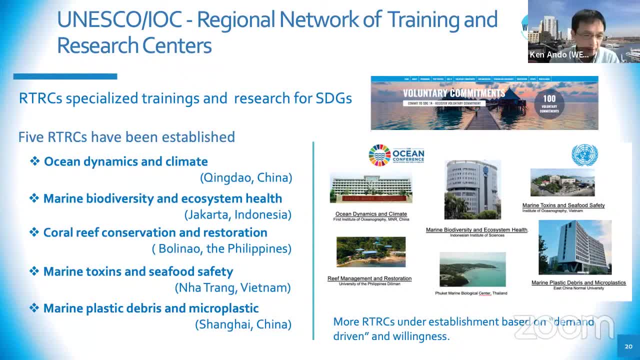 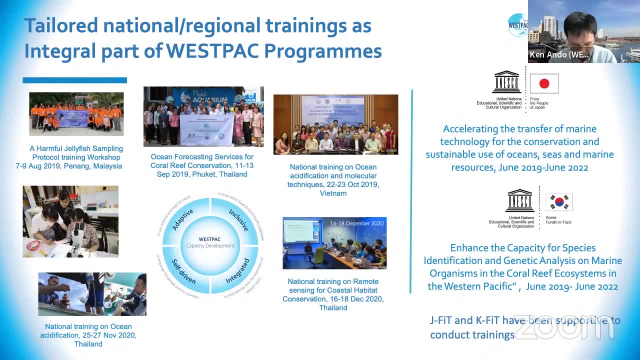 jellyfish sampling workshop was conducted and also ocean forecasting services workshop was done in 2019.. National training courses also have been done in 2019 and also 2020.. To conduct such training, for example- this is just an example- Japan and Korea have been. 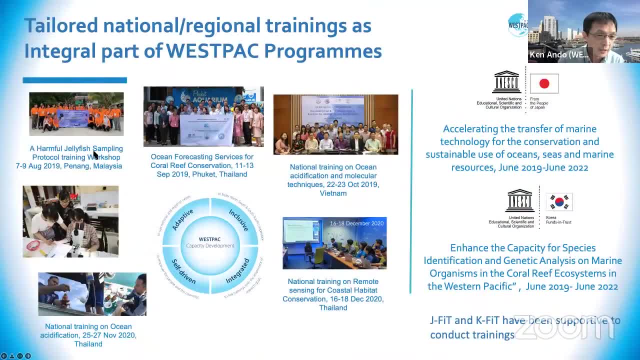 supported via each funding trust to UNESCO. This is the final slide of my talk. So in my talk I introduced the activities of UNESCO, IOC and Westpac And also I introduced several Westpac programs and working groups which are associated with biodiversity observing network. 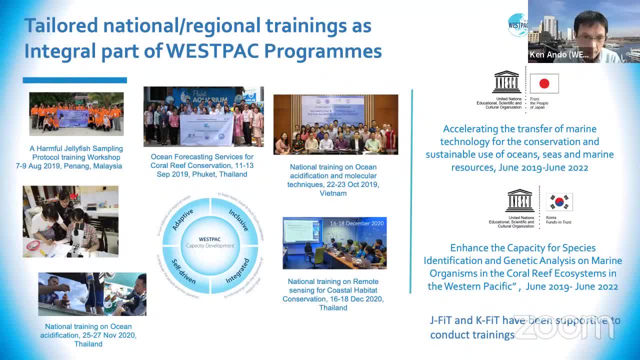 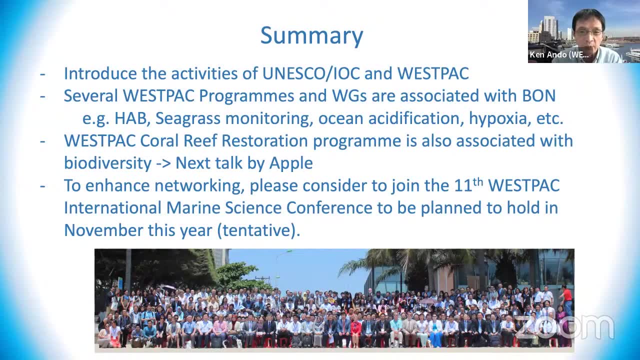 And Westpac's coral reef restoration program is also associated with biodiversity, I think. So I always talk about the HAARP project, And it is, of course, important to enhance networking in these regions. So we're going to have the 11th Westpac International Marine Science Conference. 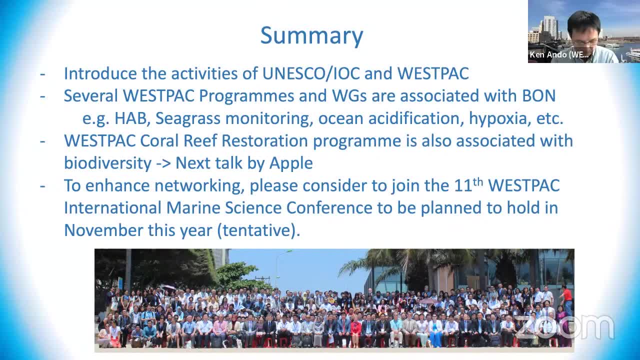 probably this year or next year, So please join to this International Marine Science Conference also. Thank you very much. Thank you very much, Dr Kentaro Ando, for a very informative and interesting presentation On the IOC Westpac activities, particularly relating to marine biodiversity conservation. 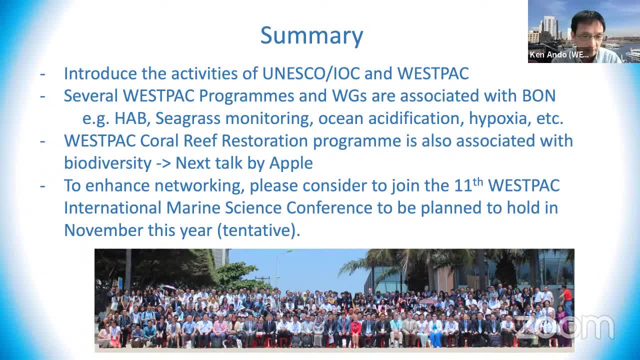 we appreciate having this kind of presentation that highlights the contribution, the huge part of the IOC, Westpac, especially including your commitment in being part of the nation's goal in achieving the future that we want and the ocean that we want. So thank you for that, Dr Ando. 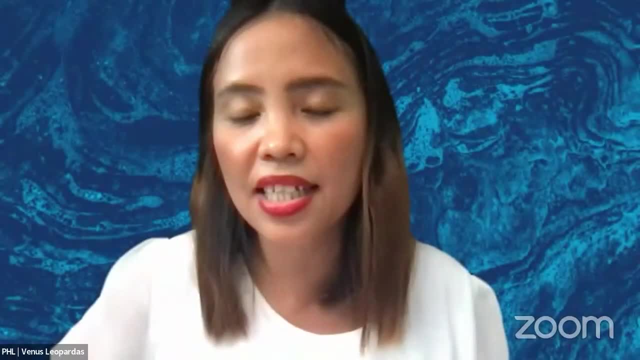 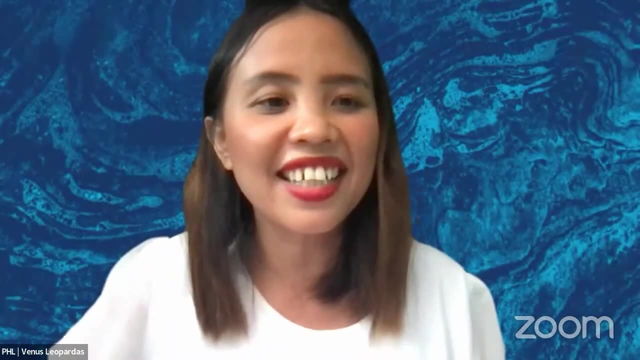 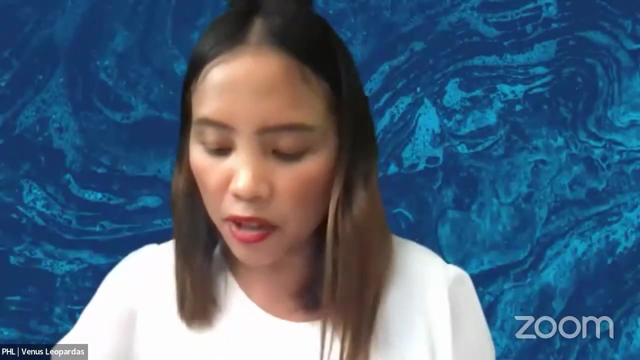 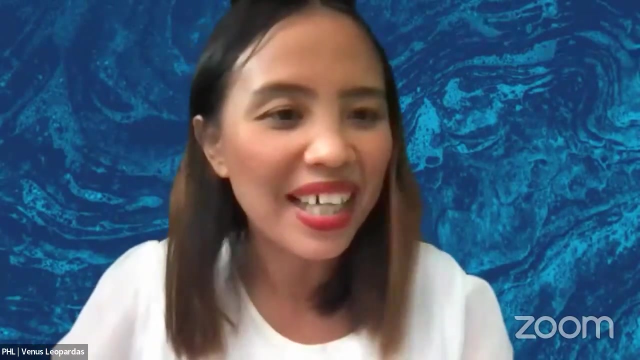 Now let us proceed to the next speaker. Our next speaker is a very known, a well-known scientist, female scientist in Thailand She is actually. she has received a lot of awards and including one of the 17 Asia Power Women of Inspiration and the UNESCO, IOC, Westpac, Outstanding. 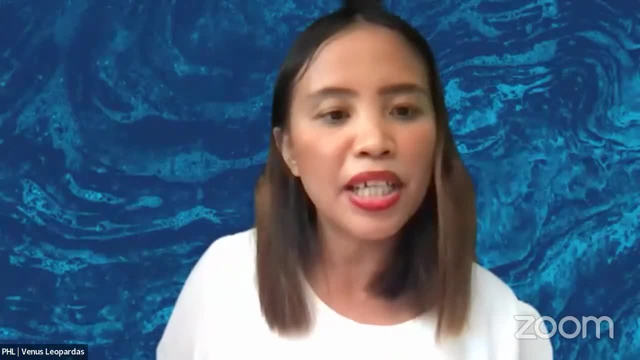 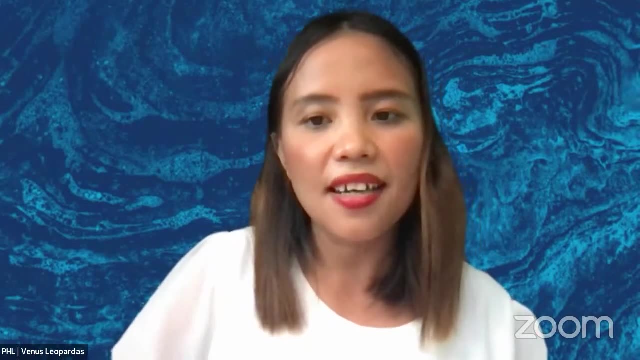 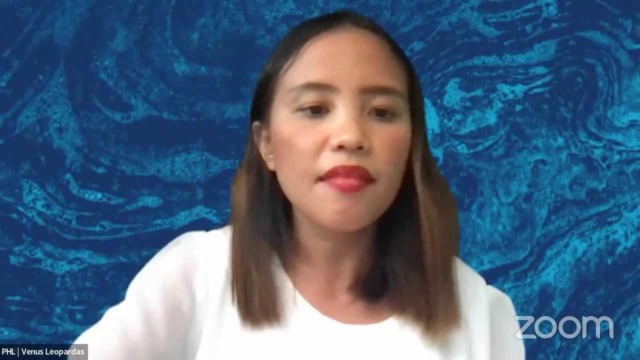 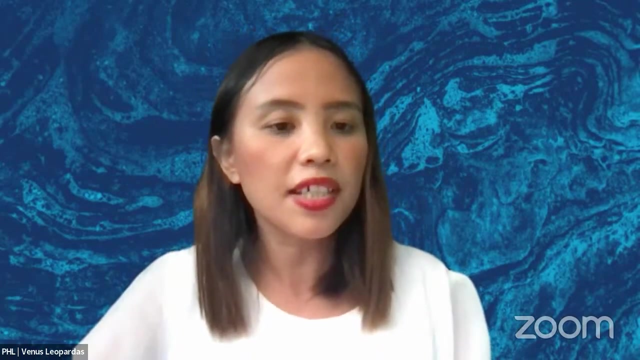 Scientist Award and also currently the Sustainable Ocean Ambassador. Please welcome, Dr Suchana Chavanek. Good morning everyone. First of all, I would like to thank the organising committee for allowing me to join this event. I'm honoured to be with you all today. Today, I would like to 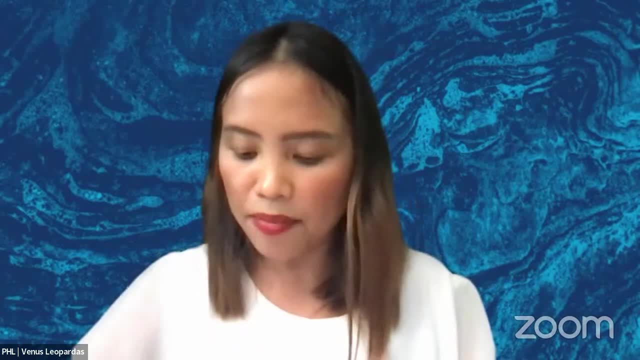 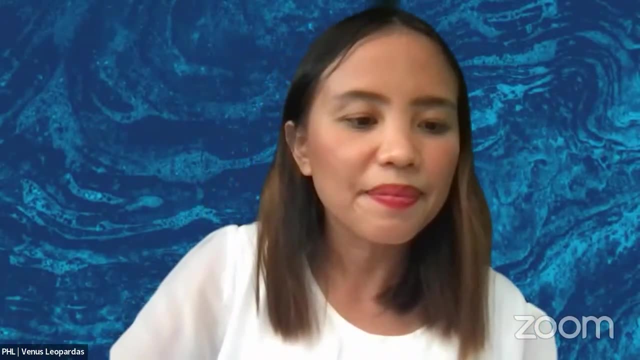 share with you about my knowledge and experience in the sector of marine conservation since 2010.. you about how we use science and technology to a better coral restoration in Southeast Asia And this presentation is a part of a coral conservation and restorations in the Western. 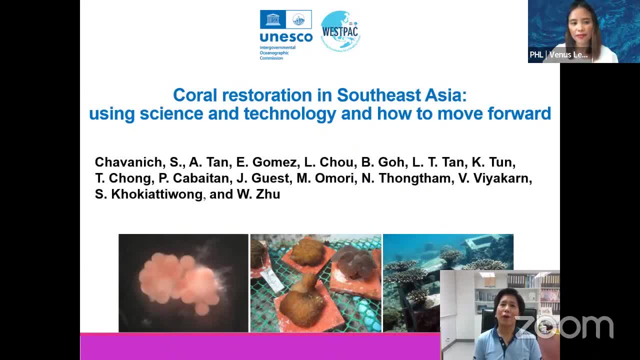 Pacific, which is under UNESCO Intergovernmental Oceanographic Commission for the Western Pacific or UNESCO IOC, Westpac, And these are the examples of the activities that we do. We do a lot of technology transfer related to the coral restorations and conservations between 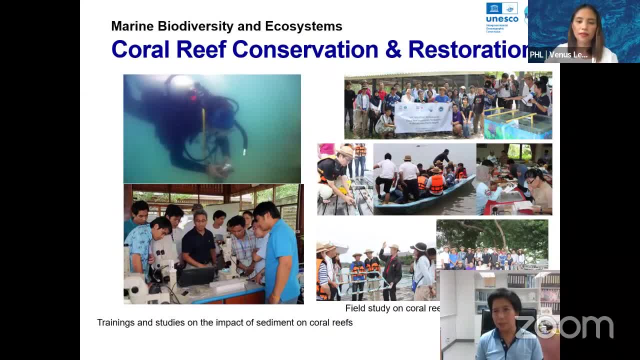 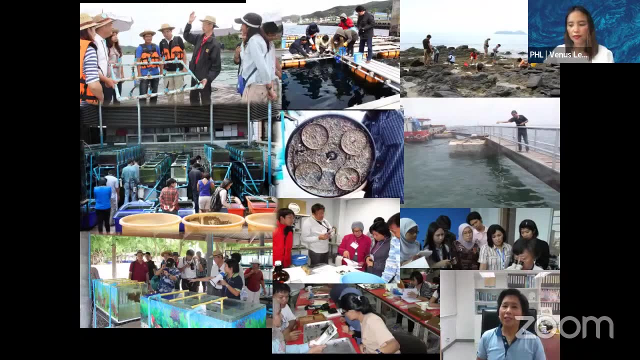 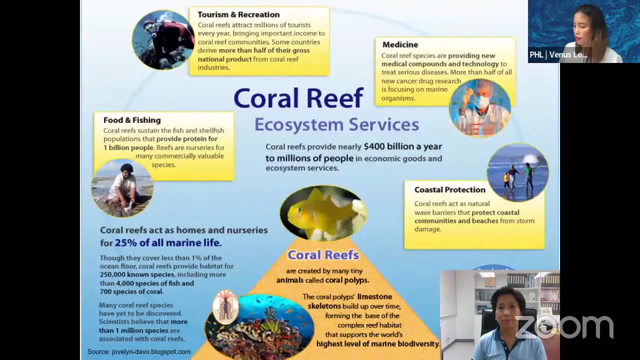 countries in the Western Pacific. As we all know that coral reefs supply a number of valuable and vital ecosystem service and goods, Such as food provisions, shoreline protections, erosion regulations and so on. However, unfortunately, coral reefs are currently under several chronic human impact, such as overfishings, pollutions, increase of the 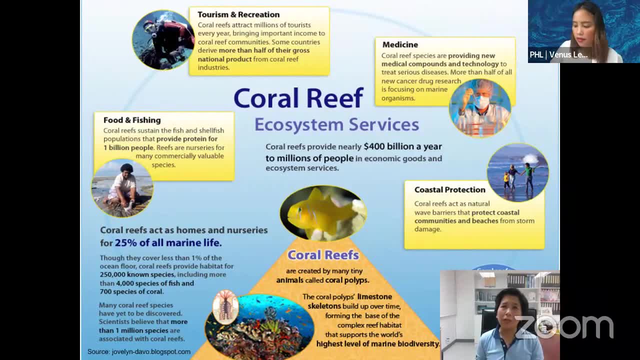 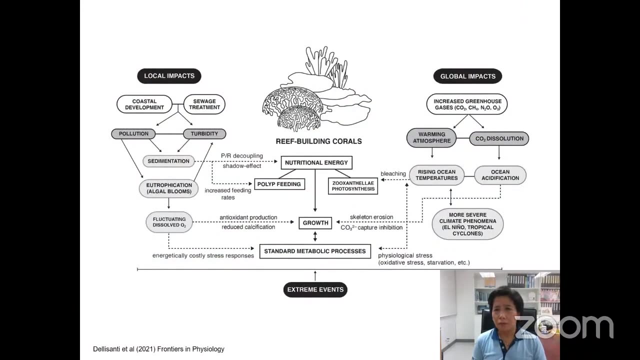 sedimentation, eutrophications and coastal developments. But actually we can divide the impact into two types: One is the local impact and the other one is the global impact. So, as I mentioned earlier, there are several factors contributing to the declining of the coral. 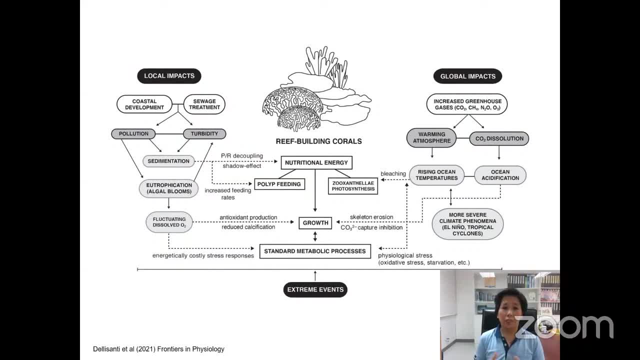 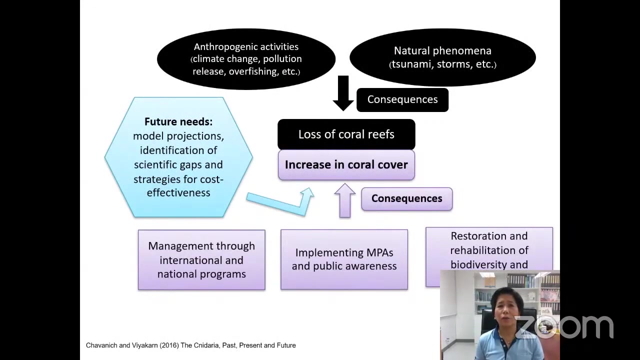 reef around the world right now, but can they be able to recover back by themselves, without help from us? We are not sure, since we are the one that create all those threats. So what we can do is to have a good management, good implementation. 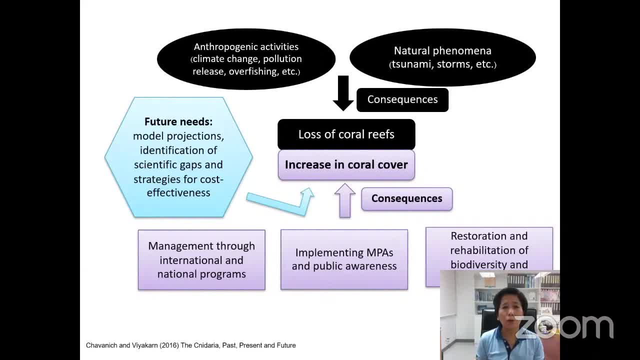 try to reduce all those threats and then restorations and rehabilitation can come. We cannot deny that many countries, particularly in the western pacific regions, in the southeast asian regions, have been using coral restorations as a tool to increase the populations of the corals in the area. 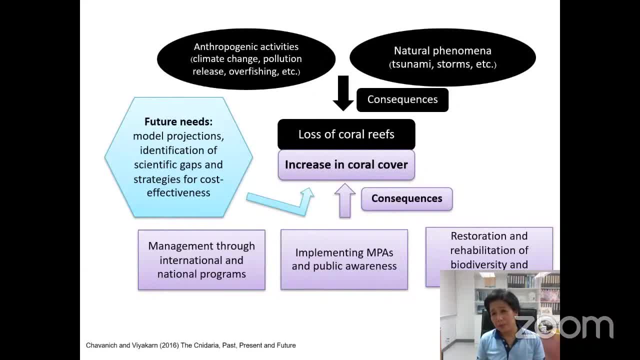 by integrating the science, knowledge and the technology together, And we hope that at least this will have one easy way to help a bit and the coral can come back, rather than let them recover by themselves, since we cannot wait for so long. 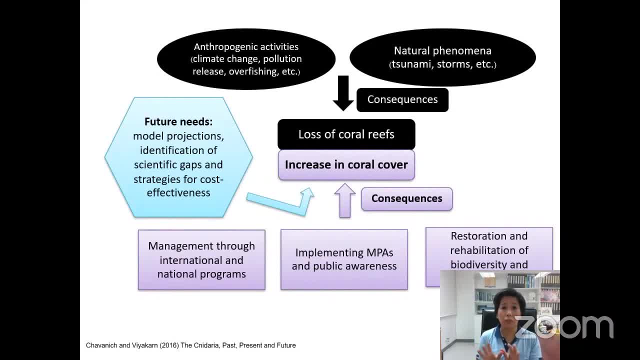 Now, particularly in the western pacific region. coral restoration is not just only for scientists, but many private sector and the company are also very much interested in this and would like to get involved, not because of the CSR or corporate social responsibilities, but they also find an opportunity for a win-win situation. 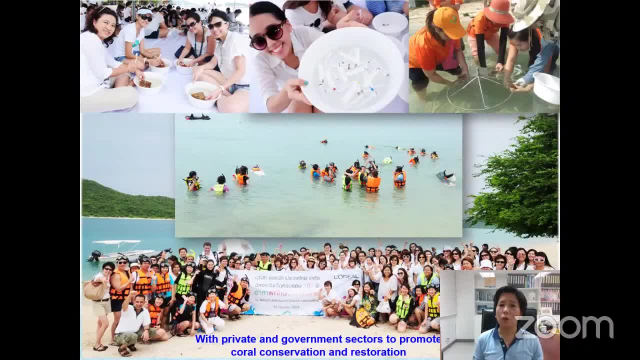 Now I would like to talk a little bit more about coral restoration in the western pacific region. I would like to share with you a bit more on detail about coral restoration technique in the western pacific region, particularly in south asia regions, how we use science and technology together for a better coral restoration technique. 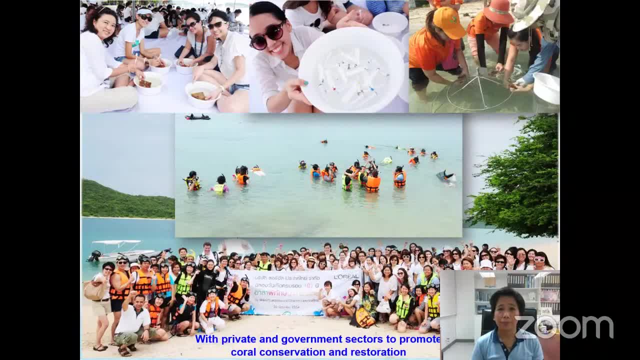 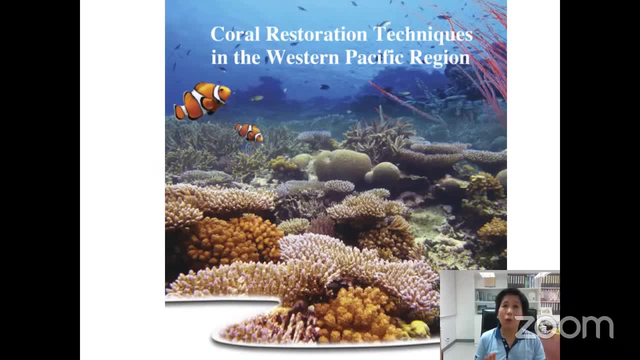 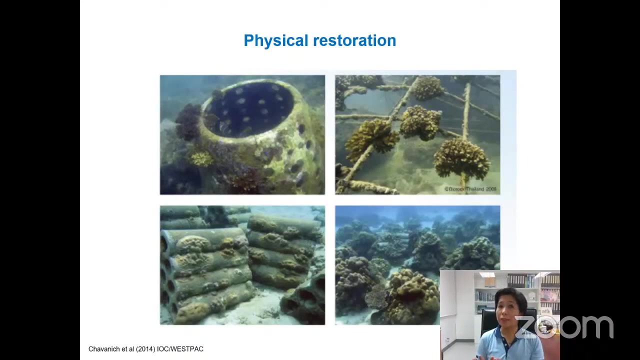 Physical restoration is one of the popular techniques in south asia regions. Physical restoration is defined as a repair of the reef environment from an engineering approach. Artificial reef creation is a common technique used for this physical restoration in the south asia area. Various artificial structures, for example rock, concrete like reef ball ceramics like 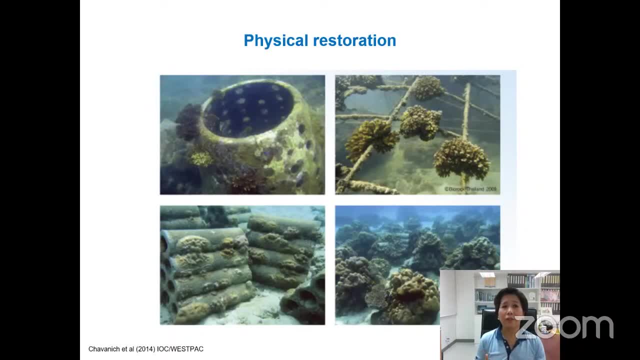 an eco reef or a carbon steel structure like a bio rock can be restored from looking for conditions. Artificial reef creation can be think of as repairing the reef environment from an engineering approach. Different artificial structures such as bones, likehing or pitton, like United Harbors DRC珍 using ceramic angle, certainly create disaster on the reef as part of coral restoration. 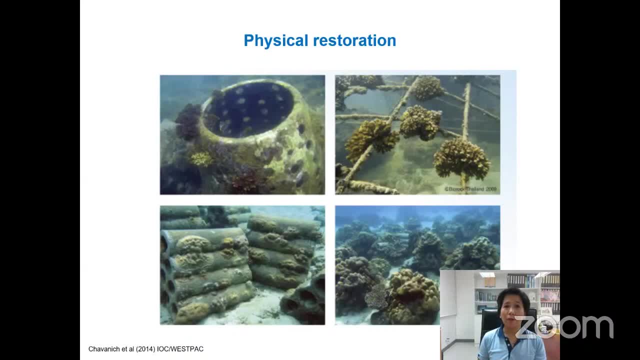 or different artificial structures, such as bioref hairstructures, can also repair the reef as part of coral restorationings directly found in the Religion skills industry. using physical restoration techniques, structure like a bio rock can be seen around these regions. This is also one of the most common techniques using in Southeast Asia regions, both flat. 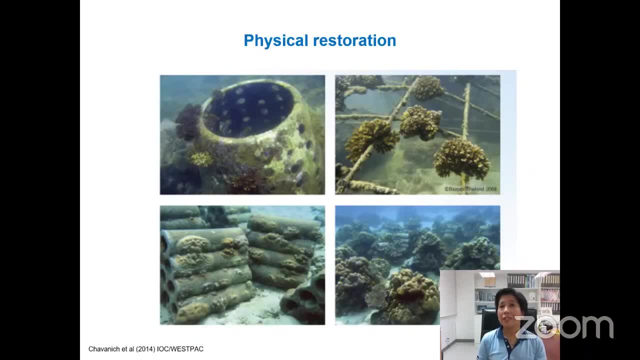 man and nutman can be used. So for this, asexual propagation is a quick and simple technique for rapid restorations of degraded leaf with a limited impact to the parent's colony. So this technique actually is good and is suitable when the donor source are available. 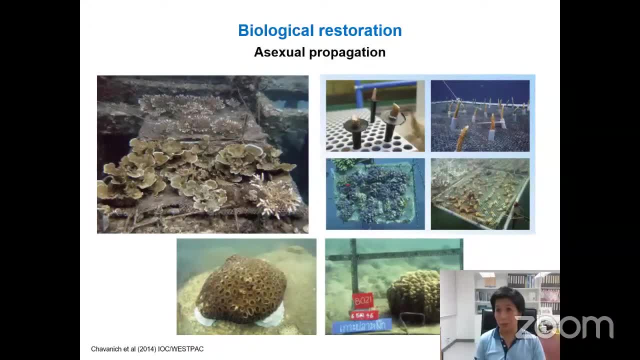 and when the resources are limited and high level technology or technique are not available. Another technique of biological restoration is sexual propagations. For sexual propagation it had been started in Southeast Asia about 10 years ago. In this technique there are several techniques that can be used. 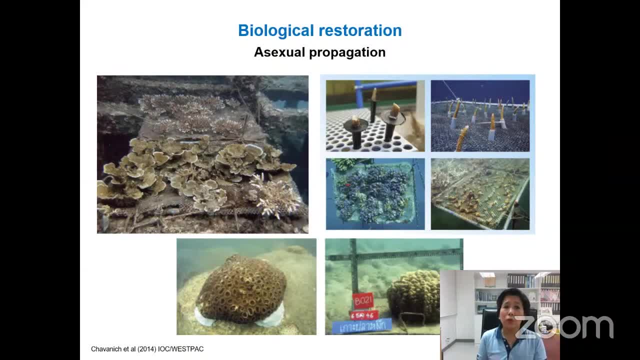 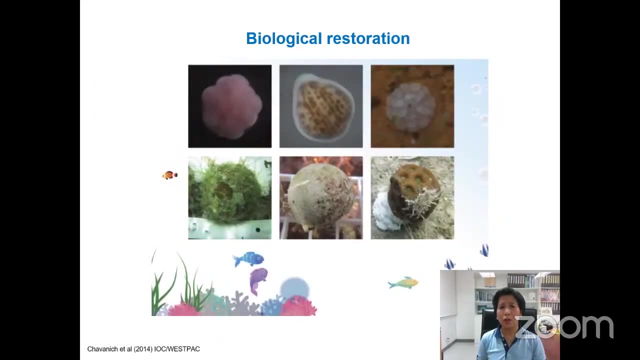 For example, there is a technique called biopropagation. In this technique, we need to consider the need of the land-based facilities for producing the larvae and their subsequently survival as an attached juvenile coral that can be out-planted to the natural leaf later on. 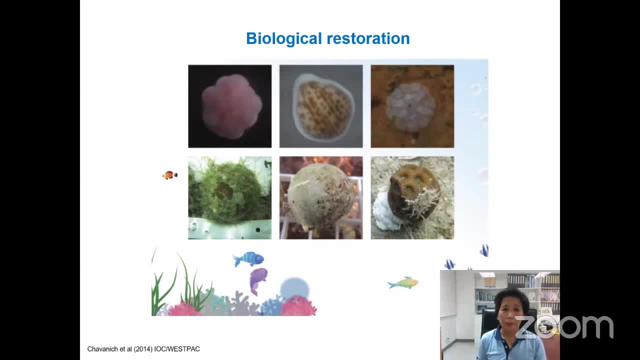 So when we're talking about sexual propagation techniques, how we do it is not really as simple as asexual. So what we do is that we have the biopropagation technique, We have to wait for coral spawn and then after that we collect the coral eggs and sperm and